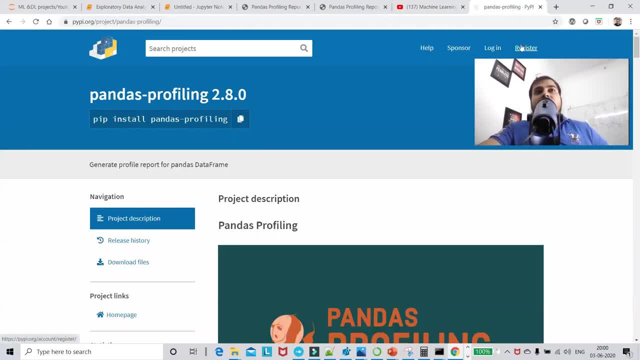 ways basically to do the reverse engineering Now. Pandas profiling is a wonderful library. This is an open source at all right, And if this is able to do an exploratory data analysis by just taking the data set, why not? We do the reverse engineering for this particular. 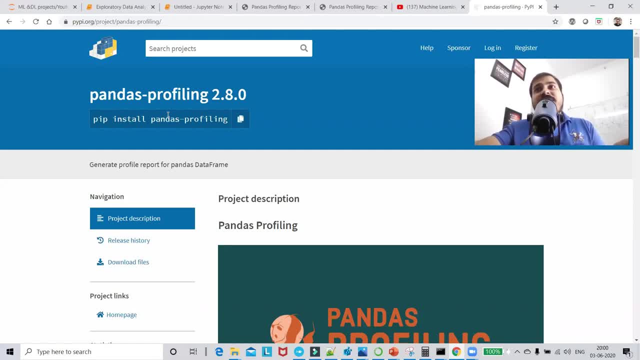 library, like what output it is generating. By that, we can definitely understand how. what are the actual steps required in the exploratory data analysis itself? Now, to begin with, what I'm going to do is that I'm going to show you two examples I'm going to take. 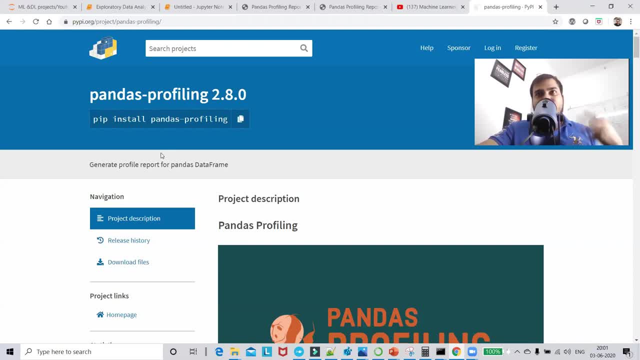 a set which does not have any missing values and another data set which has some kind of missing values, And I'll try to use this Pandas profiling to do the exploratory data analysis And you will be amazed like within five minutes we will be getting the complete reports you. 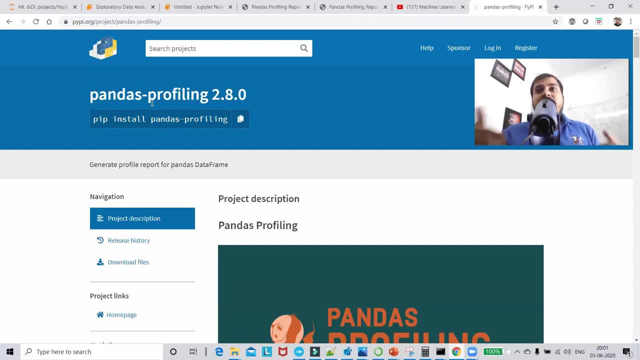 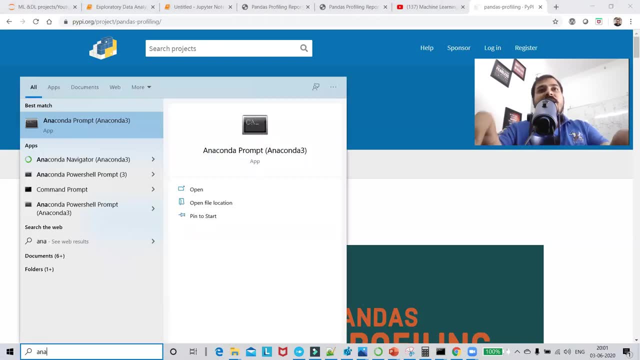 know complete report. We can also save that in the form of HTML file. So let's go ahead. So the first step is that we need to go into our Anaconda prompt. So what I'm going to do quickly is that I'm going to open my Anaconda prompt. I'm going to go into the environment. 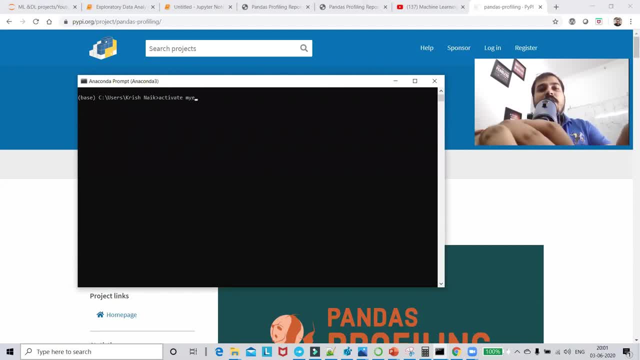 which I am an anaconda. I'm going to show you an Anaconda prompt And I'll just show it, in this case like this, And I'll just show you how I'm going to move here into my, which I am actually working on right now so that I install the pandas profiling. 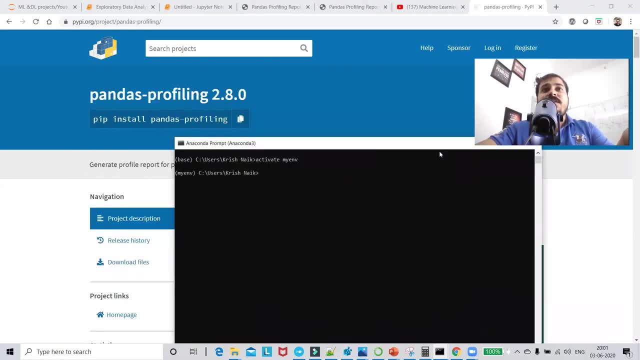 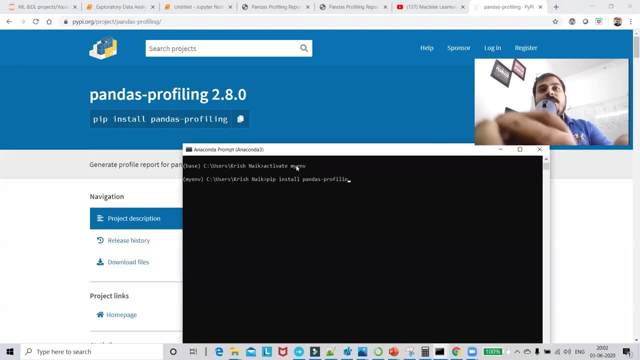 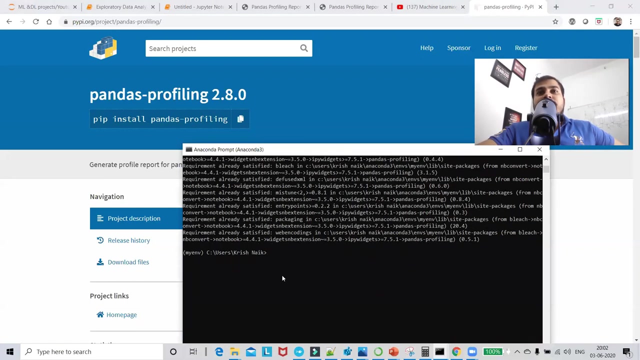 in this now, in order to install. you can see that it is clearly mentioned: pandas install. sorry, pip install, pandas dash profiling. so what I'm going to do: pip install, pandas dash profiling- right? so this is my tip: install. so once I execute this, you will be able to see that it is getting executed and over here it says: 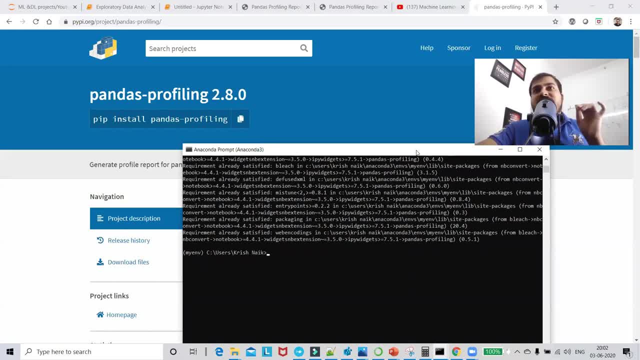 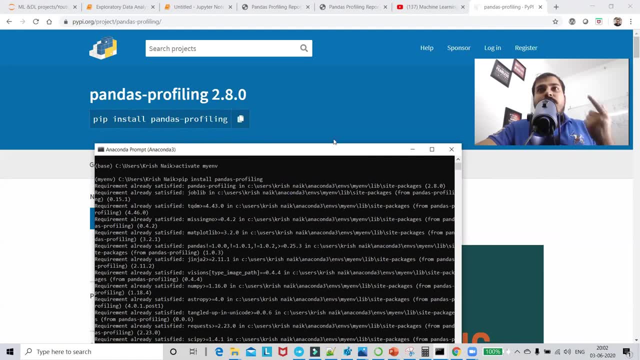 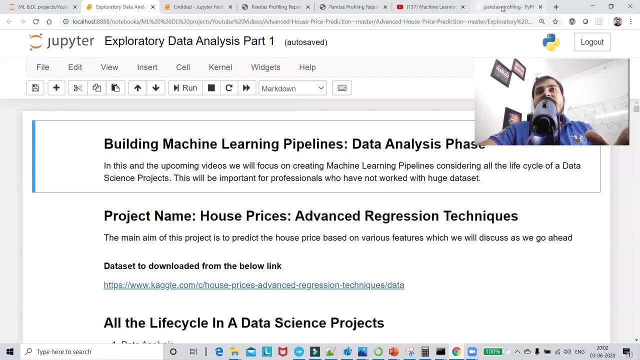 that requirement already satisfied because I have already installed aware. so this is the first step. just go into your environment where you are actually working and just write pip, install pandas dash profile. amazing, right done, your work is done. now I will go into my one of the pages or one of the videos I 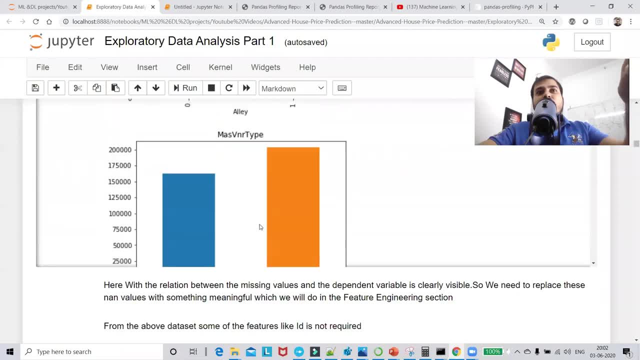 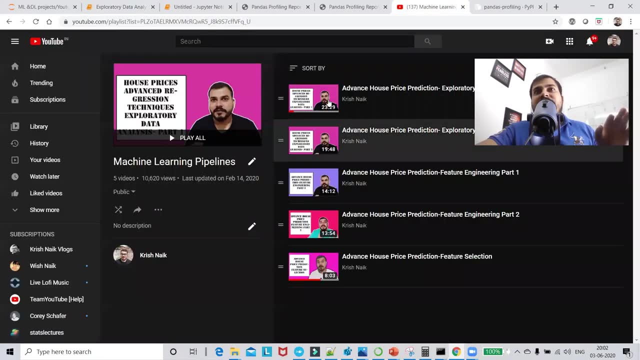 showed you over here right, and you can see that how much code we have actually written to find out numerical value, description value or missing values. again, the link for this particular playlist will be given in the description guys. you can check it out. that was the whole code you. 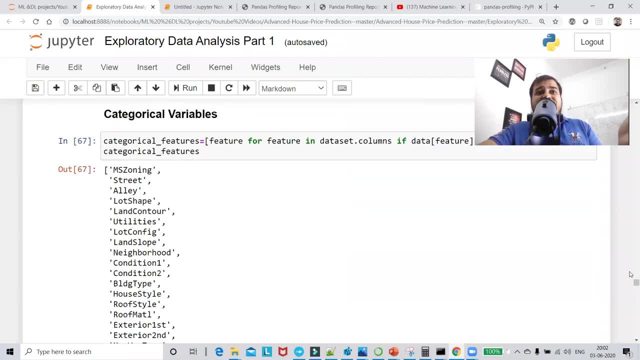 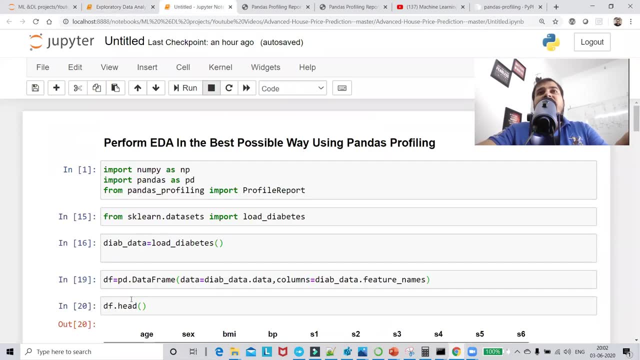 can see how much code I've actually written. you know, more than hundred lines of code are actually just written to do the exploratory data analysis. okay, so this is this is what. now? what if I make this simple by using pandas profiling. now, to begin with, guys, what I'm going to do, I'm going to import numpy pandas and 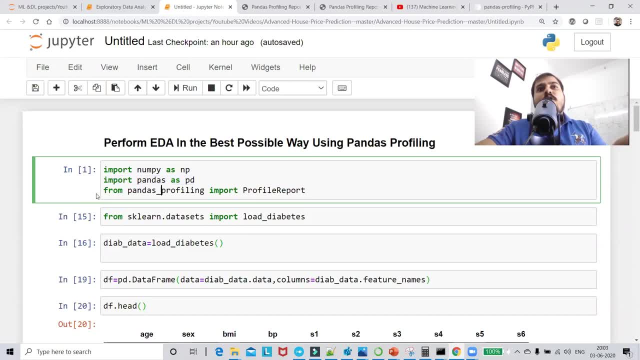 what I had installed right- pandas profiling- that I'm going to import something called as profile report. so from pandas profiling I'm going to import something called us profiled report and this report will actually display the whole exploratory data analysis report, considering the dataset that we are. 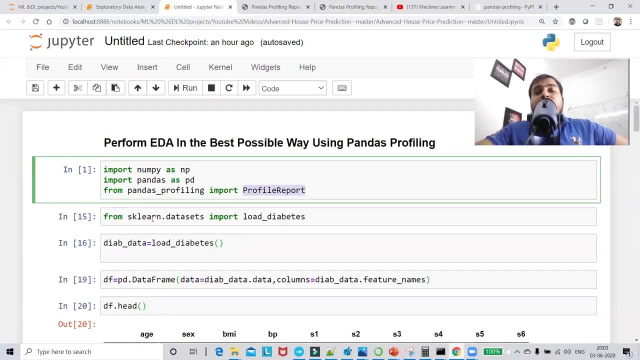 given inside this, okay. so, in the first instance, what I am going to do is that I'm going to import a dataset which is already present in a skill, and so will say a skill on dot datasets. import load underscore diabetes, okay, and this particular data set. understand, guys, one thing: this particular data set will be: 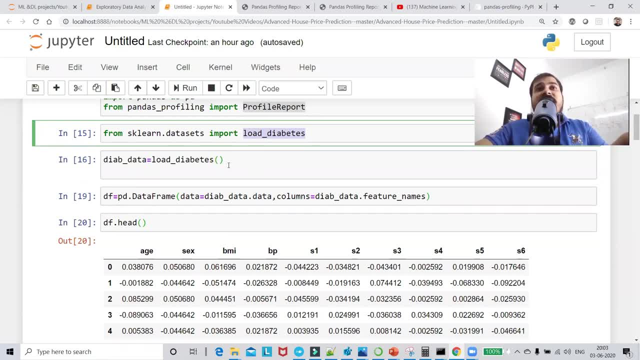 a lot of data and columns. so what I'm going to do is that, over here, as soon as I import load underscore diabetes, I am going to initialize load underscore diabetes. so as soon as I initialize this, you know I will be getting diabetes underscore data, dot data. so this, if I use dot data, it will be consisting of: 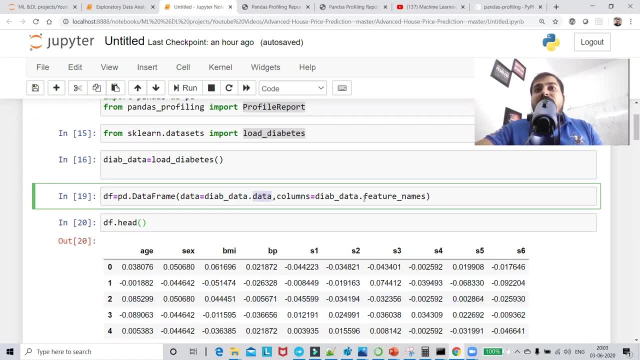 all the data that are present in that if I just go and write dot feature underscore names- you know diabetes underscore data, dot feature underscore name, because this is the variable that is getting saved right. so if I go and write dot underscore, dot feature underscore names, I will be getting all 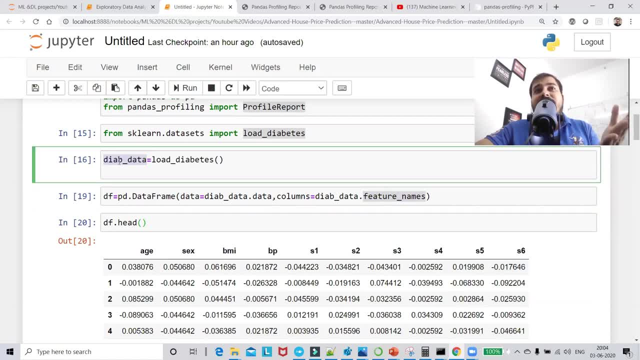 the features that are that are present in this particular data that we have loaded from the SQL and data sets. okay, then, if I do df dot head, you can see that I've combined this into a data frame where I've given my data, I've given my column. that is what is required in order to create a data frame now. so 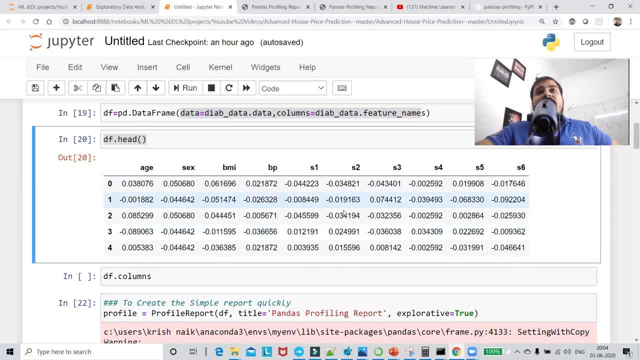 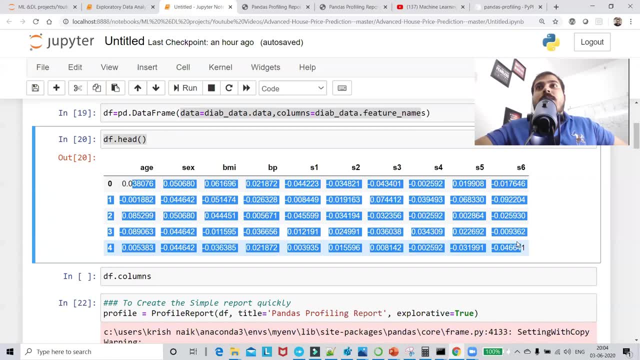 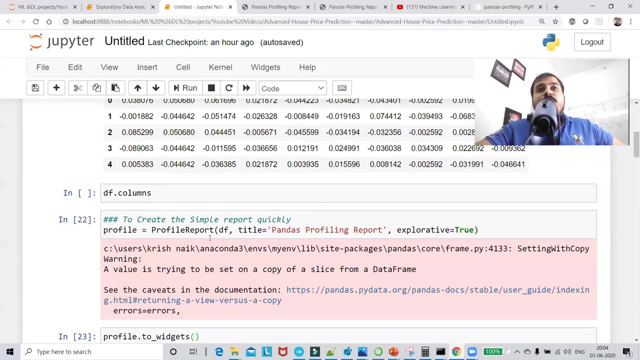 this is what is my data frame looks like and remember I have already explored this. this does not have any missing value. the data why you're seeing in this particular format is is already normalized, okay, so let's let me just and in order to execute profile report. it's pretty much simple, guys. we just have to use profile report, okay, and 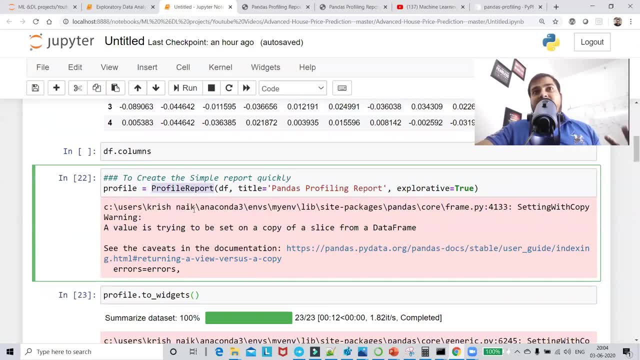 this will actually create a simple report of the exploratory data analysis. so the first parameter will be my data frame, which I have actually created. okay, the second parameter is what a kind of title you want, and the third parameter is something called an exploratory physical. to true, you just set it as true. 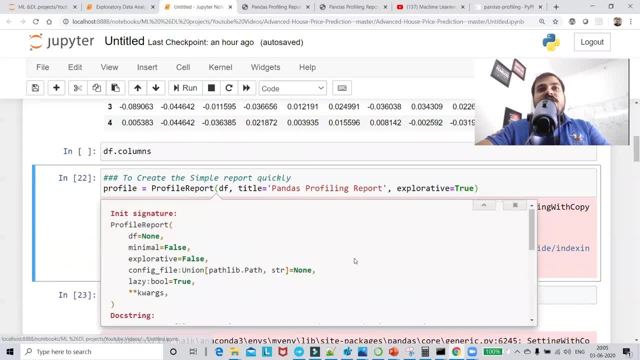 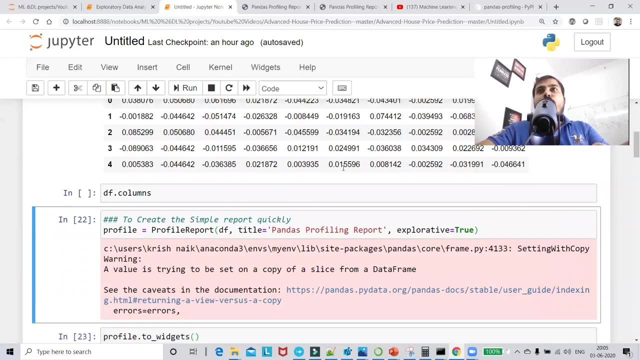 if you want to see more parameters, just press shift tab here you will be able to see all the information. okay, just before the bracket, press shift tab. you'll be able to see all the information. and if you have any queries with respect to the implementation, just go inside this particular page. okay, in this page you. 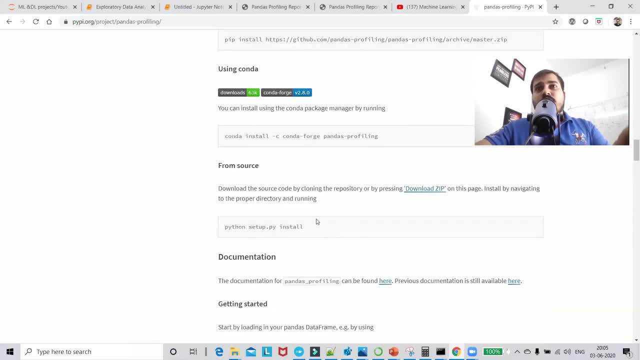 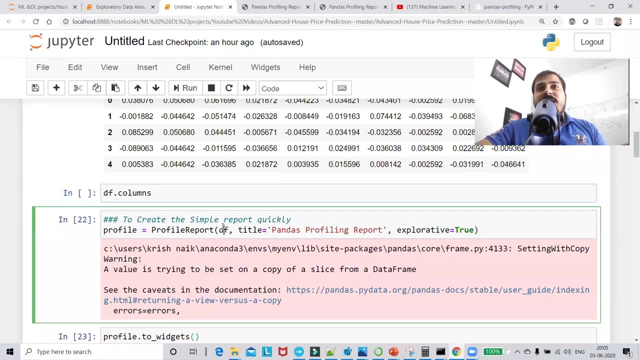 will be having all the information because, since this is a completely open source, okay, all the information itself. now, what I have done. I have initialized this profile report. I have given three parameters: one is my DF, one is my title and one is this explorative is called true. now let me do one thing. let me. 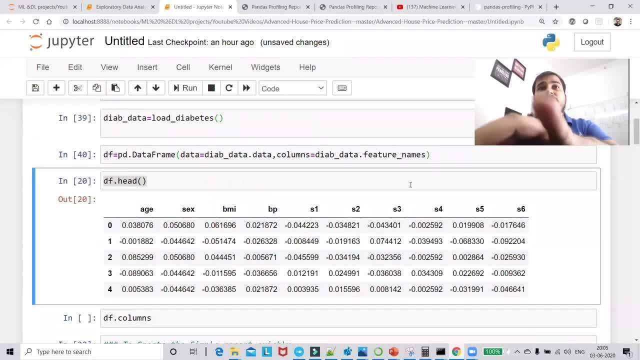 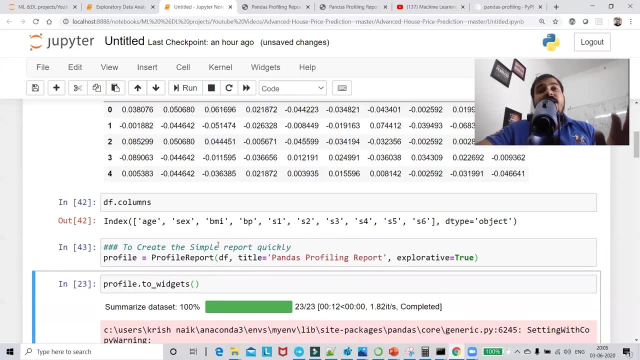 quickly execute in front of you. you be able to see that within five minutes, you know, within five minutes. not only five minutes, guys, just two minutes. you know you will be able to see that the whole report will get created. now, in order to create the report, no, you just 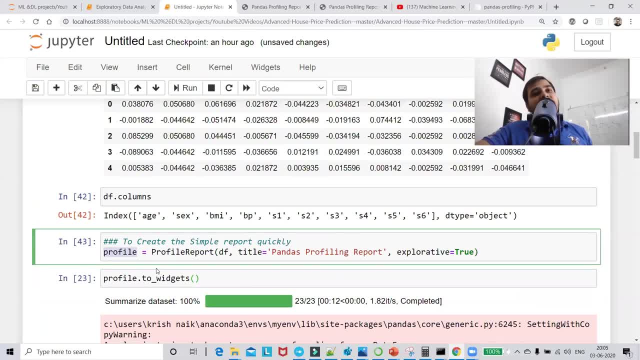 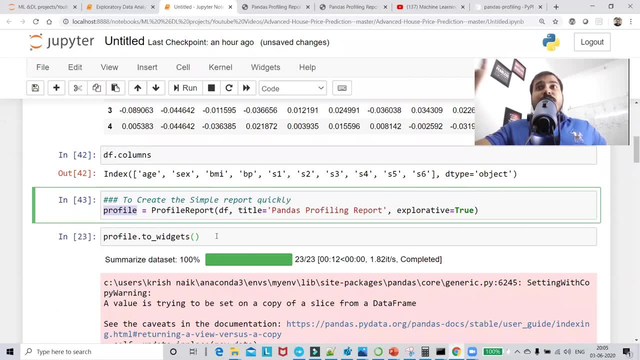 you can use two techniques. one is something called as two underscore widgets. you know, widgets basically means you will display all the report within your Jupyter notebook. the other one is something that we can create: an output HTML- no, in the form of HTML- so that we can see in the new page. so first we'll 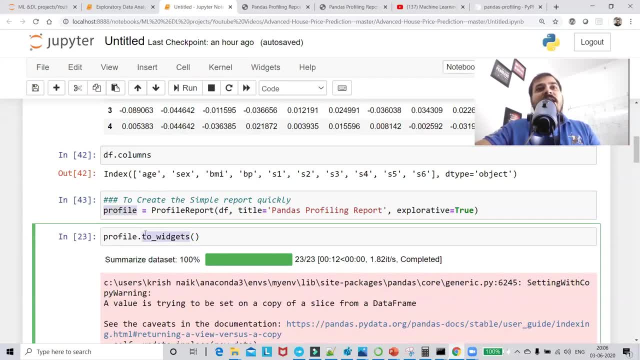 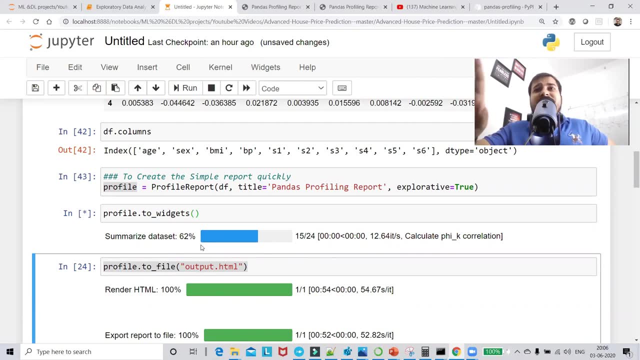 try with widgets. so over here you can see I'm just using profile dot two underscore widget. so as soon as I execute this, probably it will take. if you have a slow computer, guys, it will take around two to three minutes. I have a little bit faster computer so probably it may be within 30 seconds. this will. 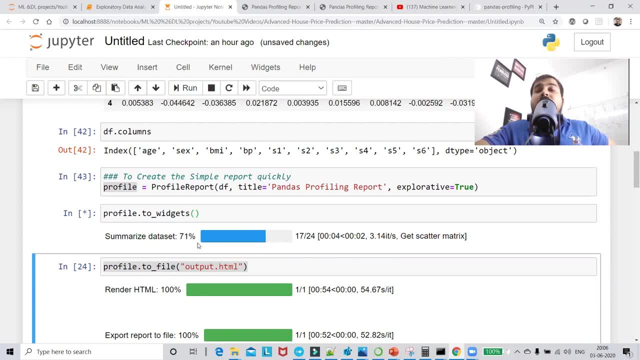 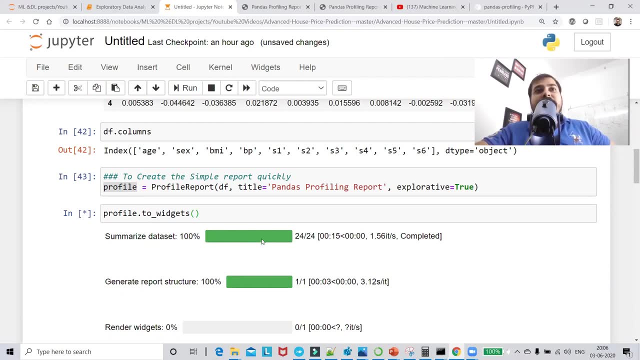 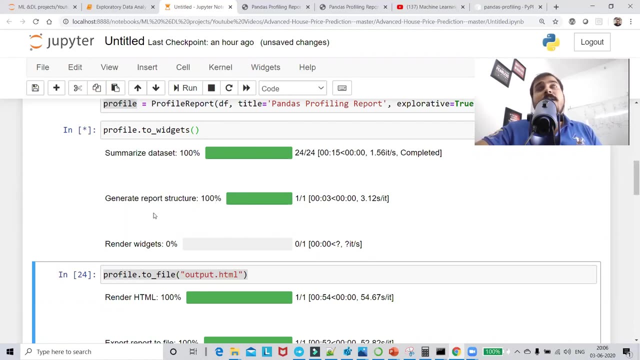 actually show you, and this also depends on the amount of data that you're having. suppose you are having many number of features. you have many number of records. that much time it will be taking okay, so make sure that you have a powerful system. if you feel that your computer is very, very slow, try to execute this in Google. 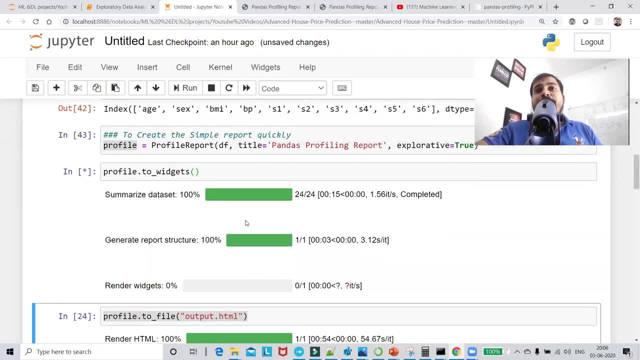 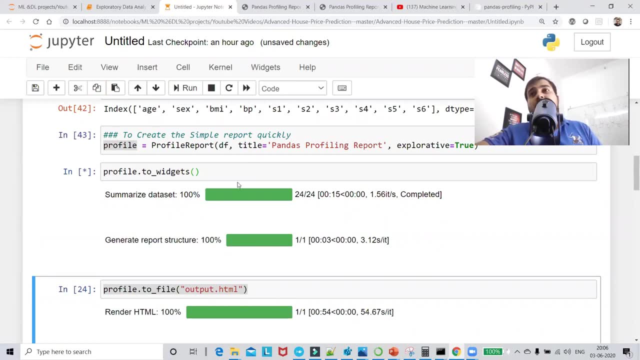 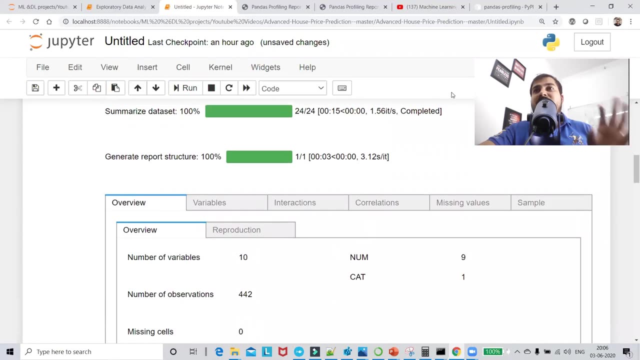 Colab. okay, in Google Colab you will be able to quickly, you know, render this kind of reports very, very quickly itself, you know. so it will be very, very much easy, and Google Colab is definitely faster. now you can see that within 10 seconds my whole report is getting generated, and it is so nice. I see this. 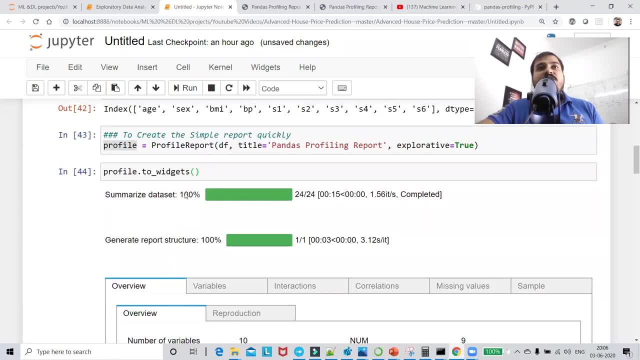 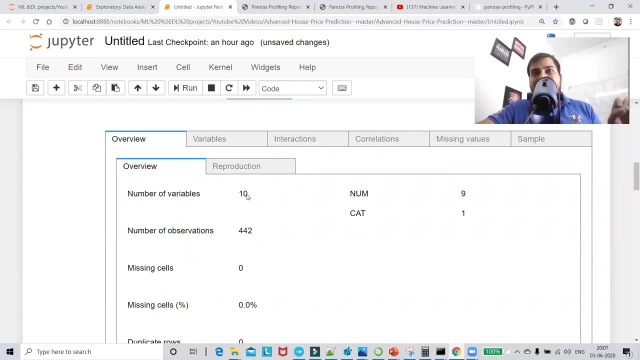 reports. it is so amazing, you know. so, first of all, as soon as I gave my data set, my data set, you can see everything is numerical value right over here. so over here: number of variables: 10 perfect 10 features are there. number of observation: 442. missing cells: 0. Mrs Nihal. percentage 0.0. 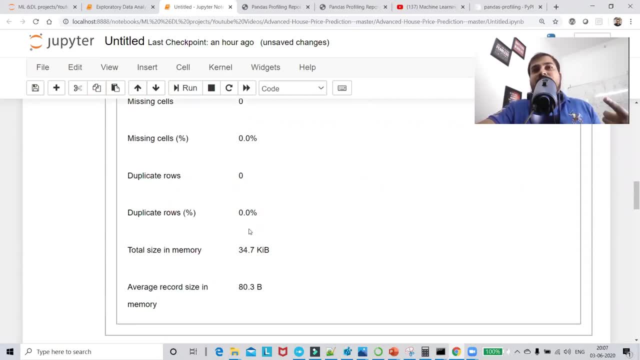 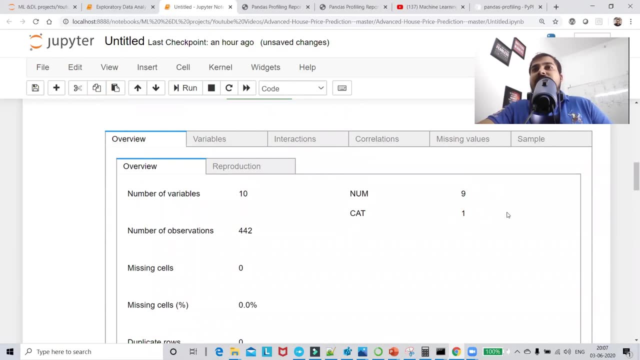 duplicate rows: 0 duplicate rows. a percentage: 0.0. total size in memory. it is also saying that how much memory it is taking in order to load that specific data. okay, numerical value, category value: everything is given. okay, then you have you. you have some of the details like: 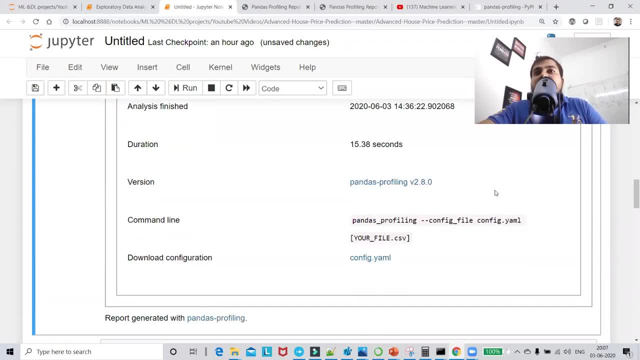 when did the analysis start? and it is finished duration version which PANDAS profiling version it is used, like: when did analysis start and this is finished duration version which PANDAS profiling version it is used. you can also do it by using from the command line and these all. 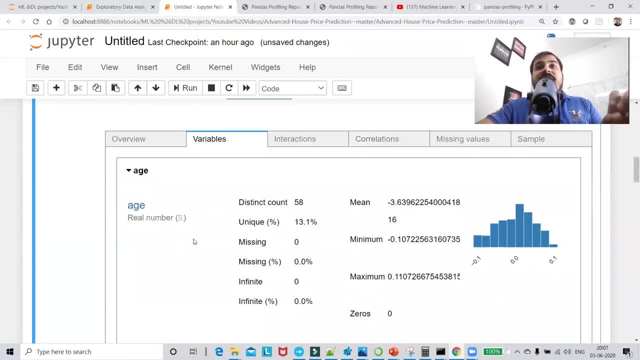 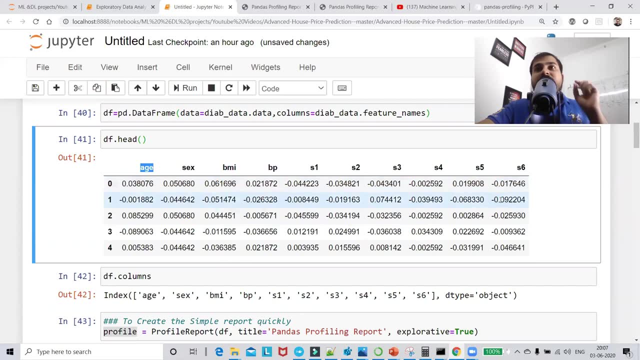 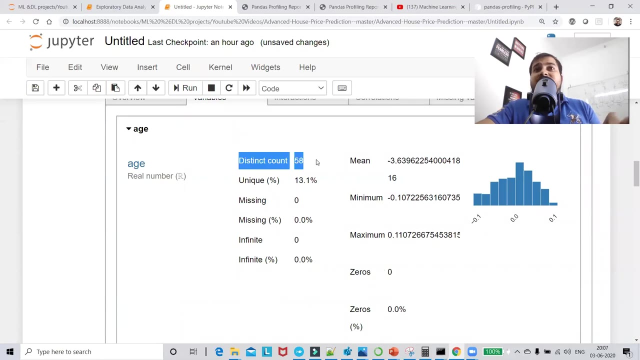 configurations are there. then we go to the variable side. now see variable also. it is pretty much amazing. for each and every variable that is present away, it will analyze- okay, it will analyze each and every variable present in the data set. so here you can see I have age over here, so age it is saying that. how many? 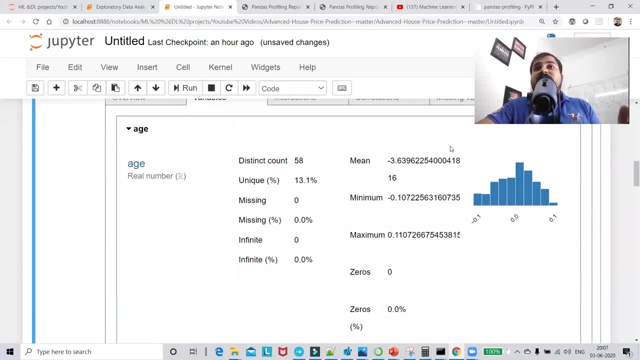 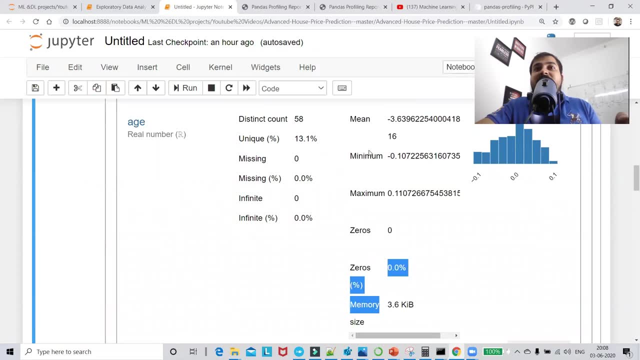 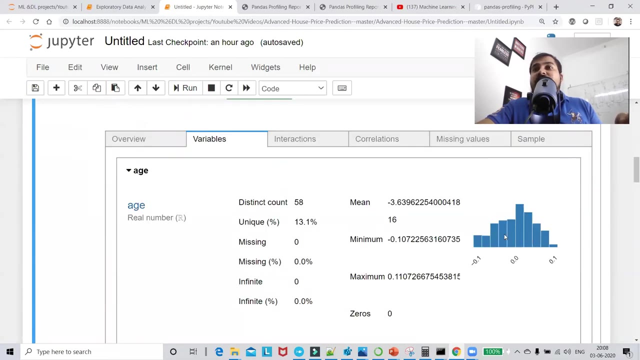 distinct records are there? how many unique records? how many missing values? everything mean mean I'm a mum, so all this information is there, right? you can see over here maximum. so we have mean minimum, maximum zero, zeros, memory size, everything are there. you can see that how the distribution is there, right? 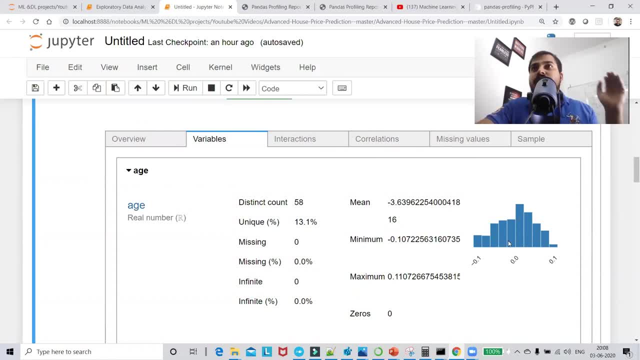 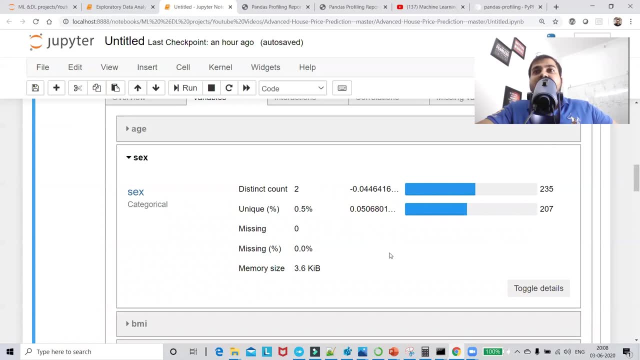 amazing distribution. you can see from what value to what value the distribution actually present, right? not only this, guys. let me just go to the next feature. that is sex. okay, now, in sex also, you'll be able to find all these informations right, and this is what it is. 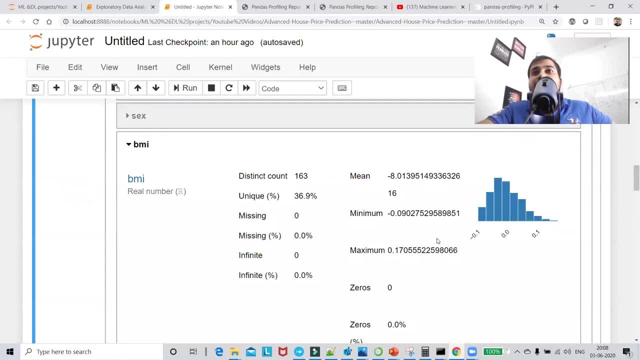 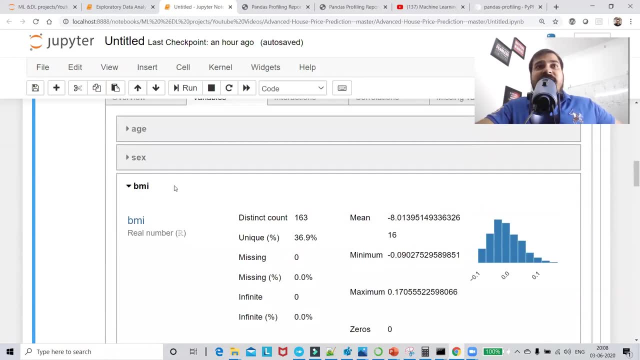 this is what it is basically saying with respect to sex. I have these values with respect to BMI, you know how it is actually distributed, how the values are actually distributed, because this is already normalized data. understand that thing, guys. then we have BP, all this particular data. just understand, guys, reverse engineering. 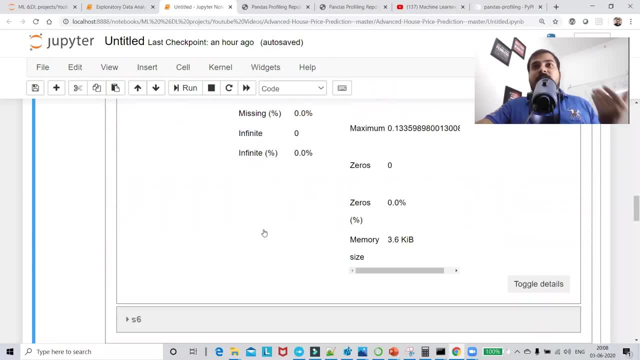 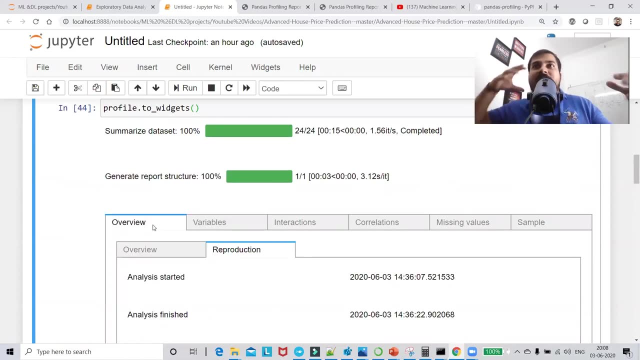 suppose you are very, very new to data analysis. right, you're very, very new to data analysis. at that time, if you want to know what all things we have to do, first of all use this particular library and do the reverse engineering technique by understanding, okay, the first state: it has found out that how many numerical 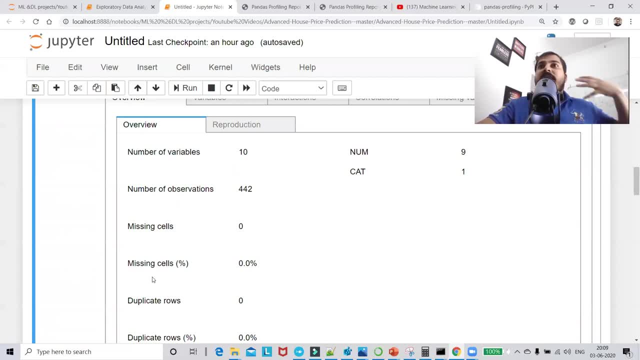 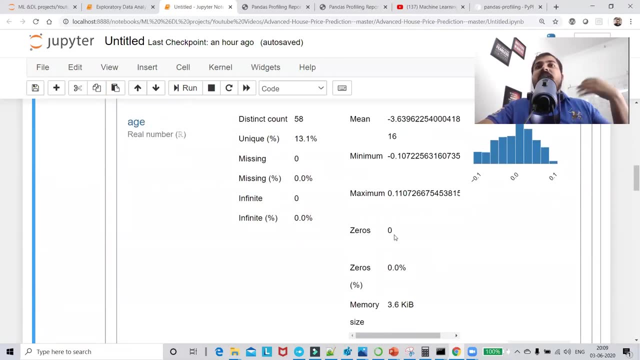 variables there? how many category variables are there? how many number of observations are there? how many number of missing cells are there? how many number of duplicate values are there? the next step you go with understanding each and every variable distribution. what is the minimum value? what is the mean value? 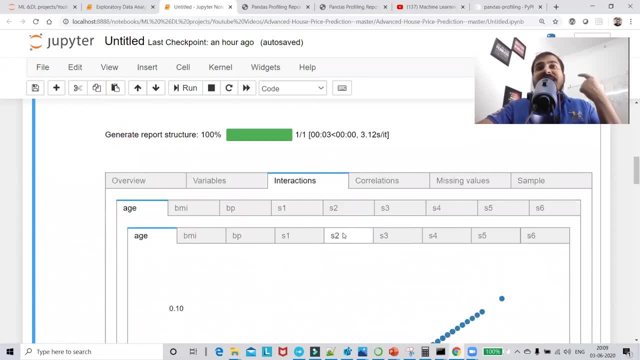 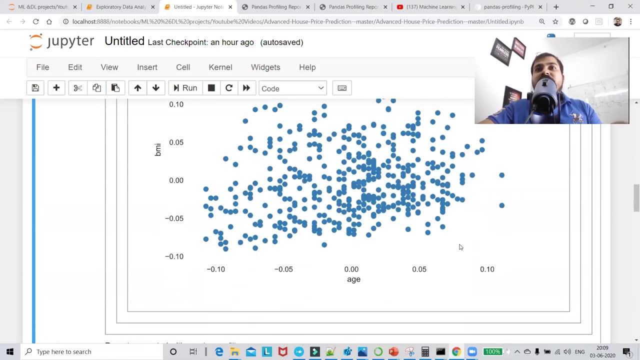 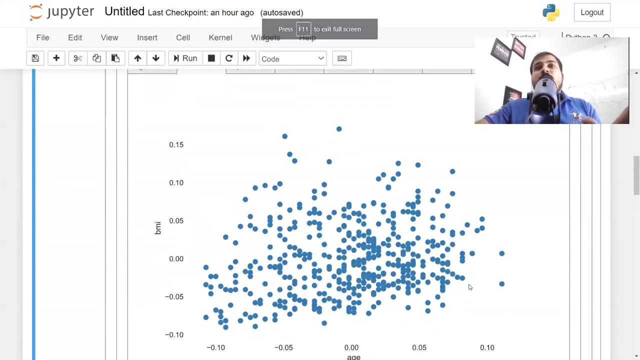 what is the maximum value? many more things. similarly, you go with the third thing. that is an interaction. interaction basically says that if I have age and BMI, how are they behaving with respect to the distribution? you can see clearly guys over here. it's an amazing- uh you know- display of information over here. right, how age and bmi? 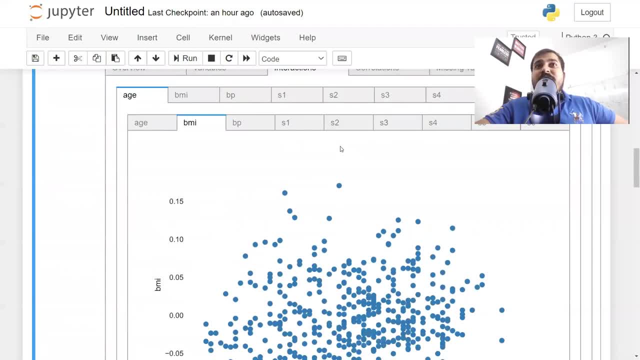 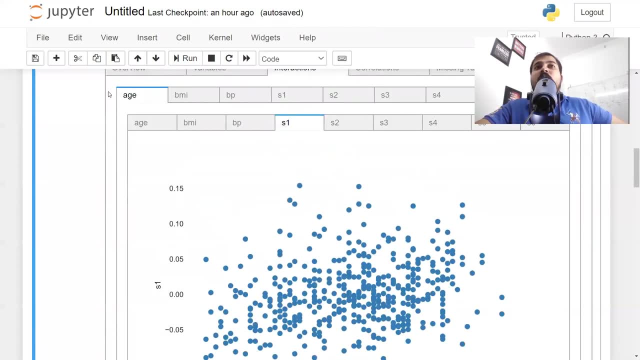 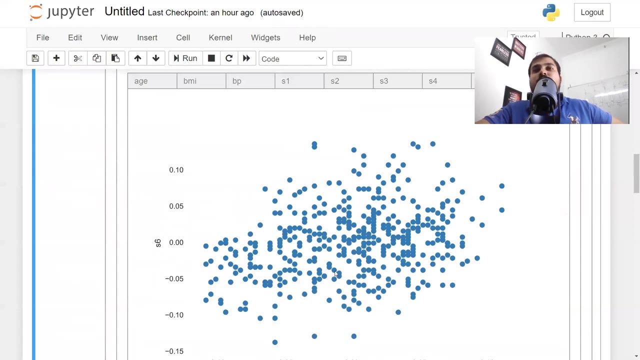 are almost correlated. how the data is distributed, you know correlation will also come now, suppose, if i want to find out age and bp- right, how it is correlated. amazing diagrams again: how age and s1 is correlated, right. how age and s2 is correlated, right, how age and s6 values actually correlated. 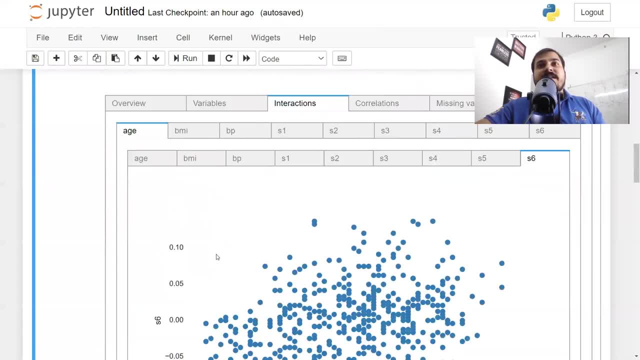 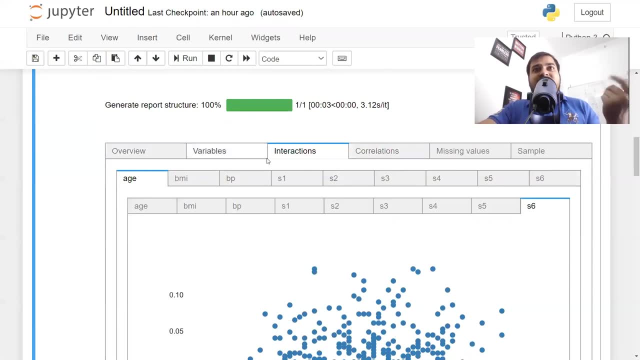 all the column information will be able to find in that particular data set itself. right now, the most important thing you know now, again, again, understand, guys, with the help of reverse engineering, after finding this, after finding this, you need to find out about the interaction which we have already done. you know, if you go and see my um, the house price prediction over there, 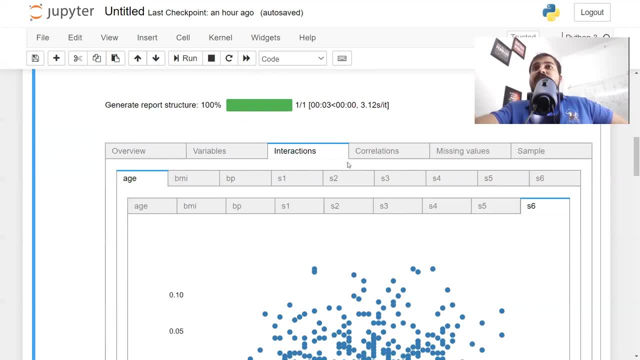 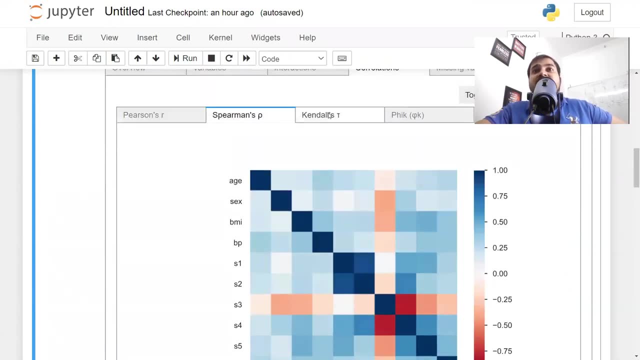 i've also done in this particular way. i have understood how the distribution is with respect to the data set. you know, then we have correlation correlation. everything is that it has applied. pearson correlations, spearmint correlation, uh, kendall's correlation, you know, uh, we have fake. 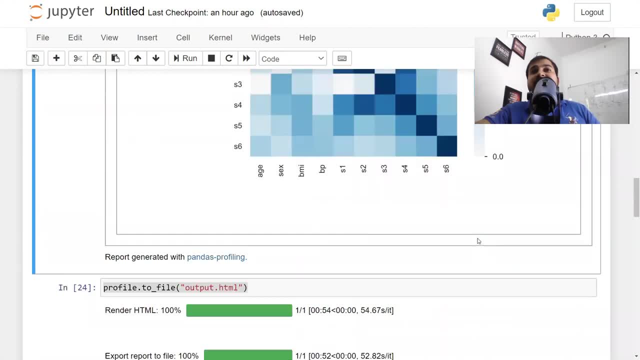 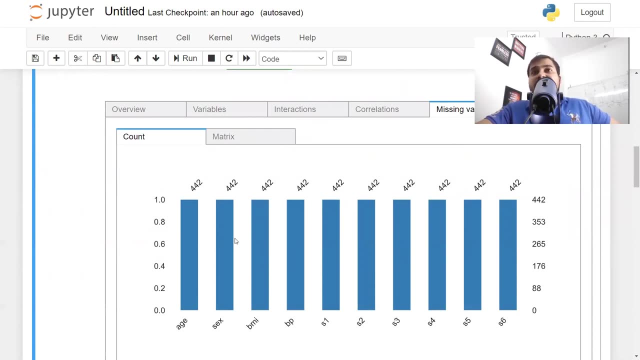 correlation. so all the different kind of correlation has been defined and it has basically made made you understand. now, what about missing values? now, this basically says that, guys, we don't have any missing value. suppose, if we had any missing values with respect to much any of the features, this would 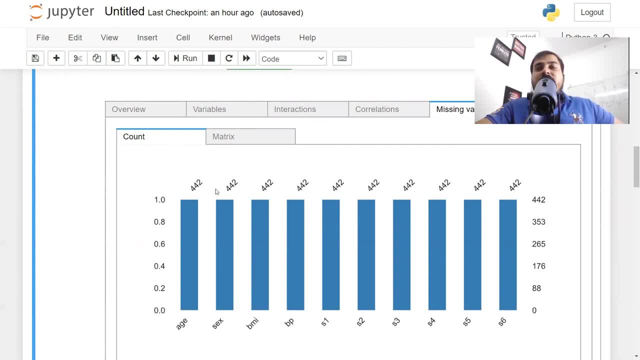 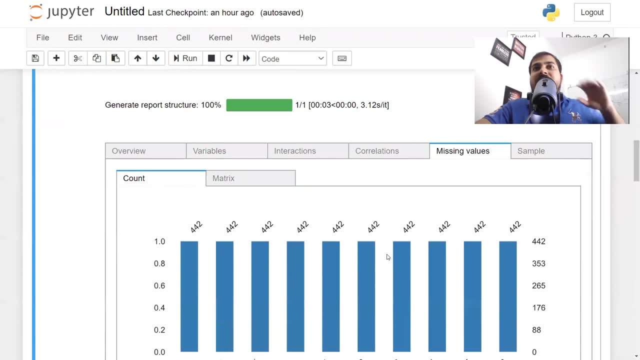 have been like: from this zero to one basically means hundred percent. from this hundred percent, how much missing values are there? like twenty percent. then it will just be pointing till point eight. okay, but right now, as i told you, i don't have any missing values. similarly, you can see: 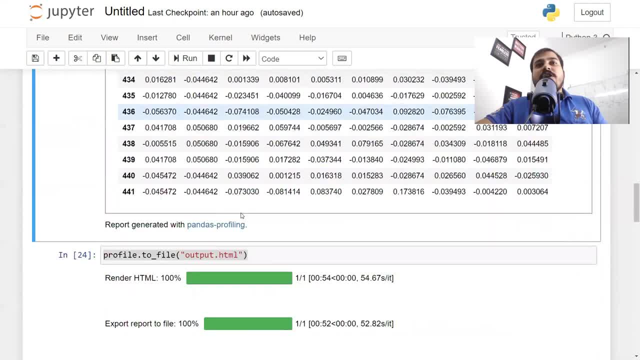 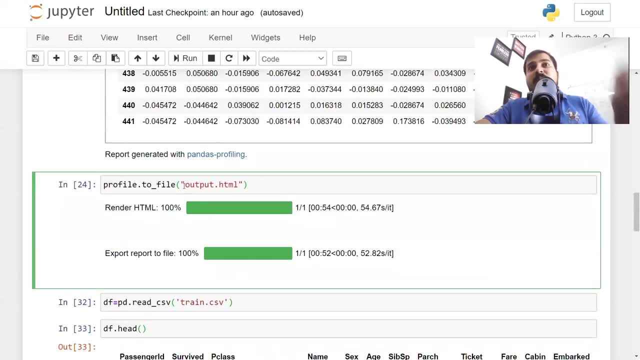 there is some sample of data set now. this is amazing. right now what i'm going to do is that i'm going to quickly create an outputhtml file for the same profile so that i can see in the web page. also. suppose you want to send this particular file to some stakeholders to understand how the 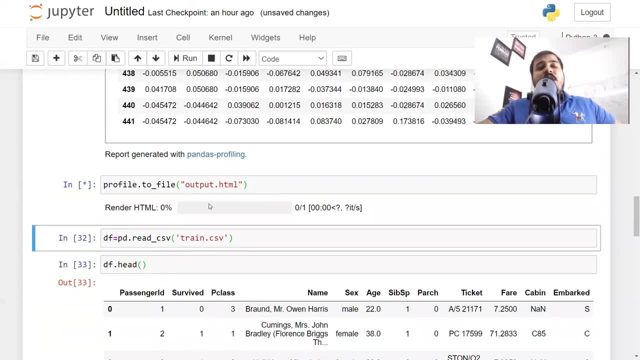 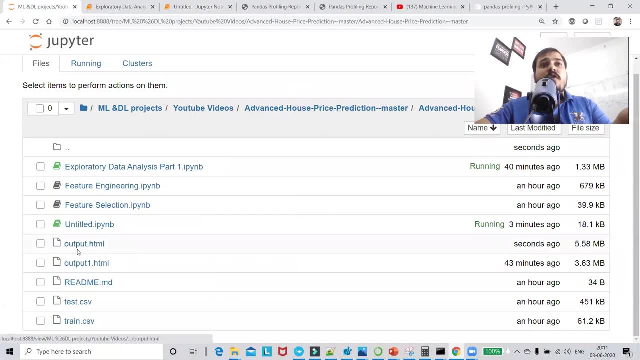 data is. i can just execute this, and probably this will also be getting executed very, very quickly, guys. uh, one thing: after: as soon as you do this right, if you go over here, you can see that there is an outputhtml, the same in the same working location. you will be able to find that, okay. so 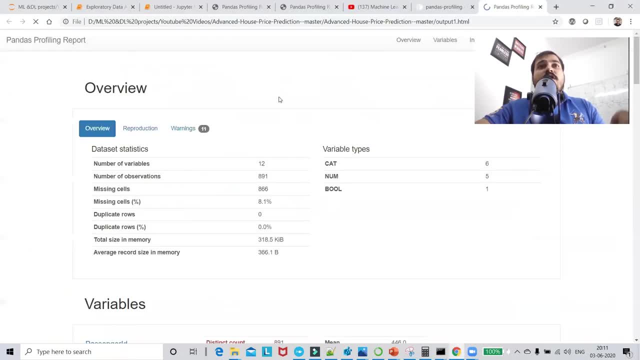 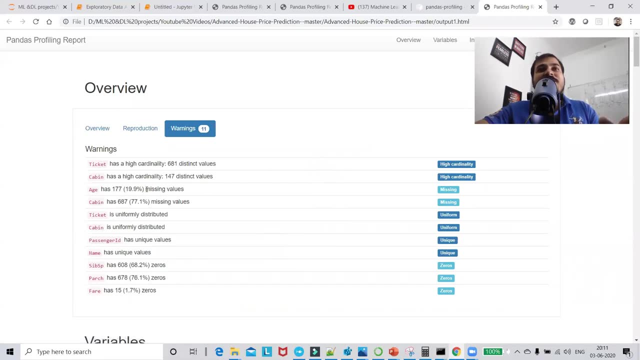 if i go over here and if i just click on outputhtml- so here it is- you can see that it is, pretty much amazingly, displaying every information. some of the warnings are also there. uh okay, uh, sorry, this is output one. let me just go to the output dot html. 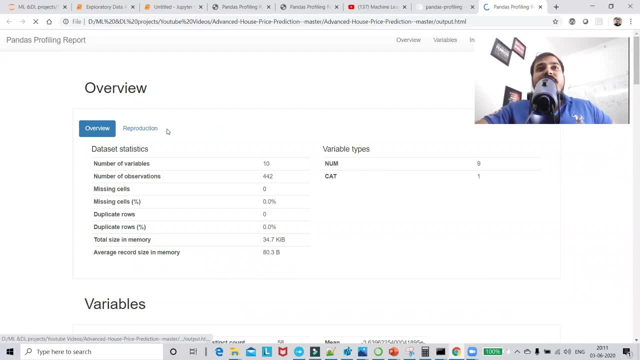 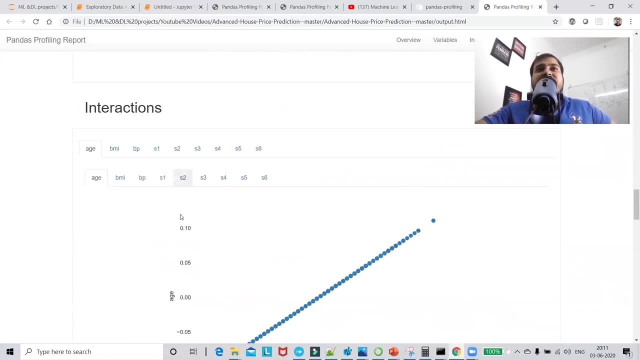 okay, so here you can see that we have overview, we have reproduction, we have variables. how the data is distributed with respect to each and every variable, same information. it is displayed in this particular manner. you can see the distribution over here in a pretty much amazing way, right is? 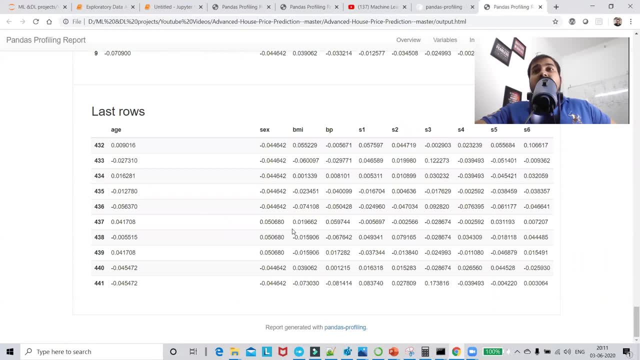 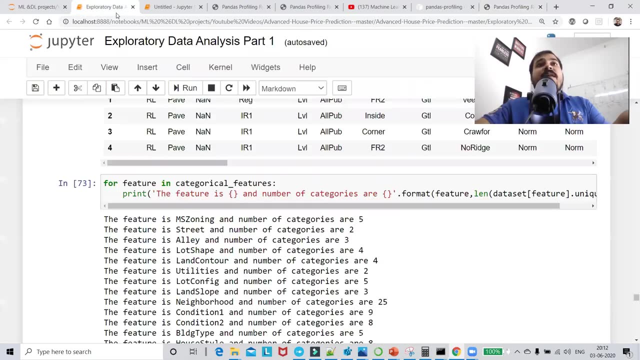 this one right here. isn't it amazing? so if you know all the steps, but just by reverse engineering this particular library, you will be able to understand so many things. okay, now what we, what i'll do, is that i'll take one more example, guys. i'll take the example of titanic data set. okay, so this is my traincsv. 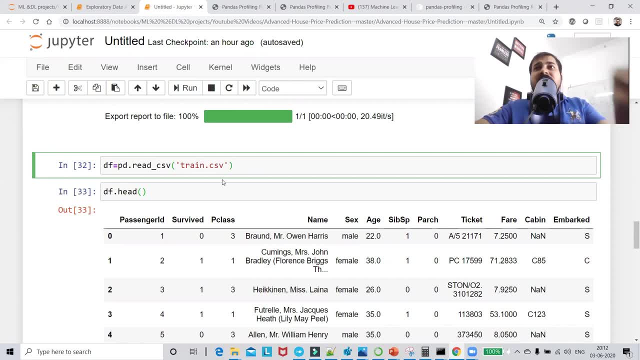 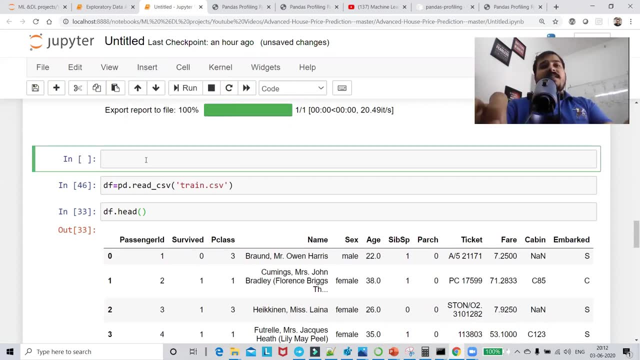 this is the titanic data set, which i have actually downloaded from the kaggle website itself, so let me just execute this. okay, so this is. i am just going to write a comment over here saying that, okay, this is my titanic, you know, okay, and i'm just going to make this as a markdown so that it looks. 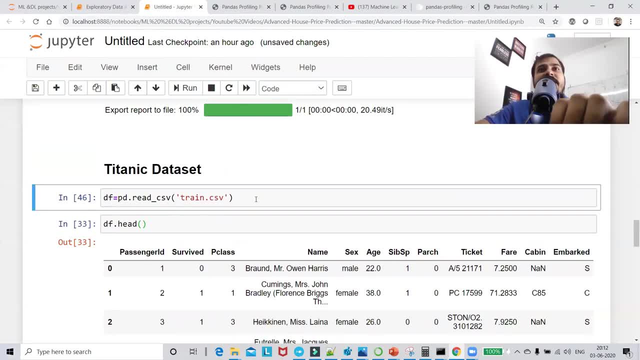 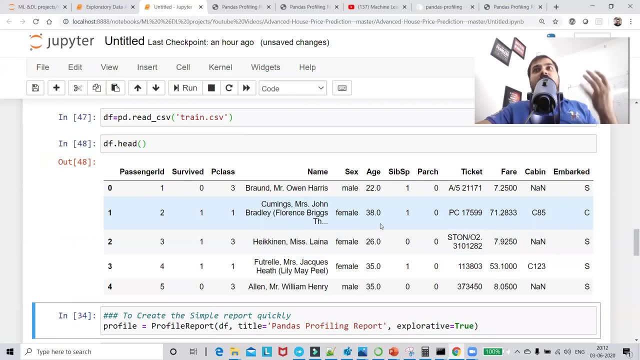 tighter so that you can also refer, you know. so i have my train data set, so i'll go to execute. this is my dfhead. why i'm taking titanic dataset, guys? because here in the titanic dataset we have a lot of missing values, you know. so it will be amazing to see how the report is actually generated again. 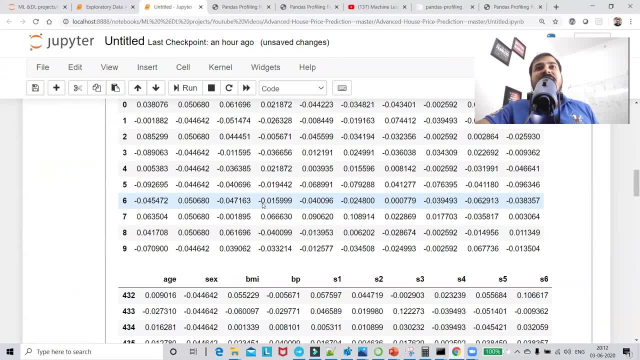 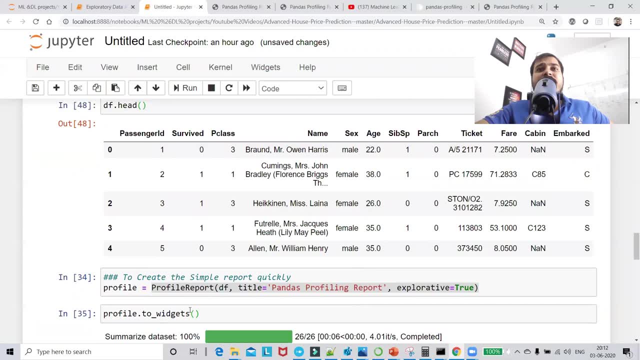 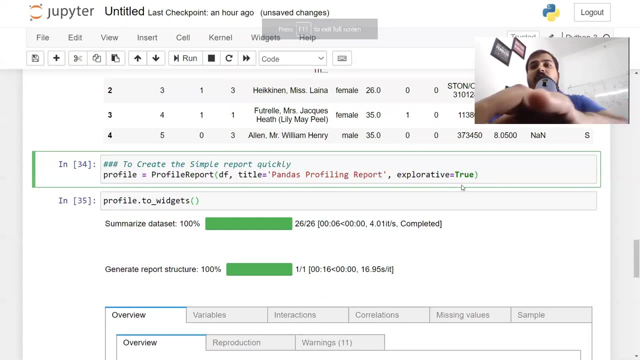 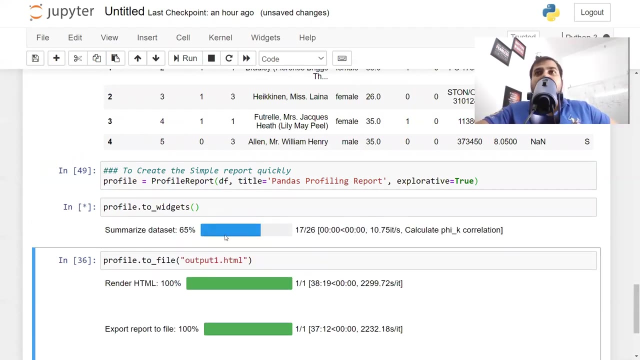 the same code i'm going to use for the profile report. that is the class that our library that i have imported. this requires two to three parameters. you that you can also give just one of them. i've given one for our draft, okay, in this case, for this part, here for our. 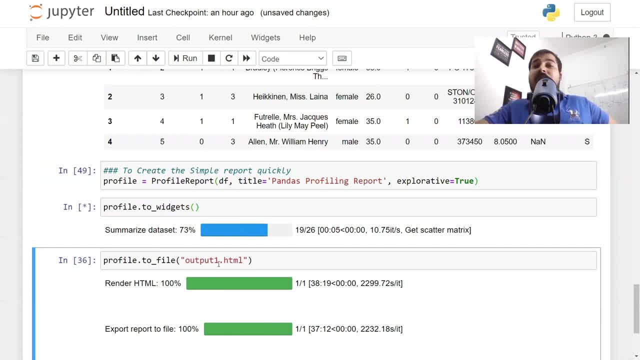 eth error. this is using the dfhead, so i'm giving here. okay, so our project is df. right, here we have a df. we can put that liquid type here. now our ник will look at the torrent for this and then from there we are going to be creating everything. the result: for now, i'll just make my event. the UI officer is up here, okay. and i'll do this. okay. so once again, спасk smart project that i have put in my shadow here. so that is df. okay, so i've given df. you can see over here i've given df, i've given title, i've given explorative is good to do, so let me just execute it. after this is executing, i'm just going to use first fault two. so this: 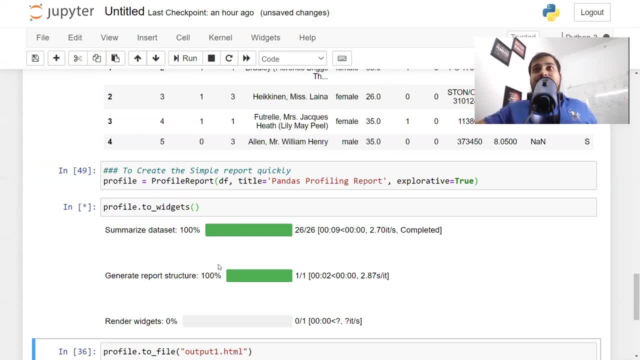 will again probably take hardly 10 to 15 seconds, and then you will also be able to see a lot of information, guys, and if you don't know what are the steps, use this library. get to know all about the steps, what is actually required, right, isn't it pretty much amazing? 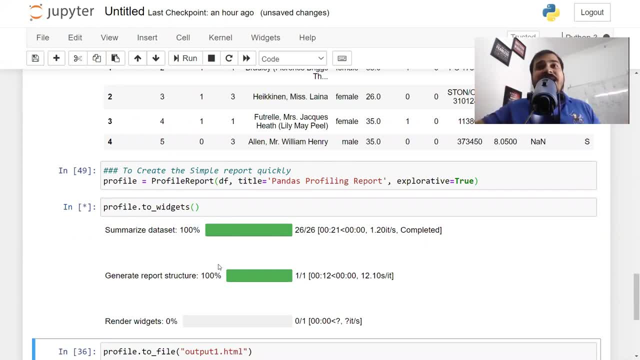 because you are able to do everything in front of you, don't require anybody's help, right? and then, if you want to do manually, you can also try doing manually by just by googling things like how to do this, how to do that, you know how to. 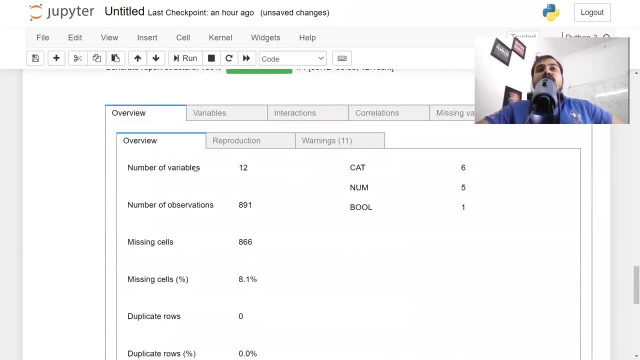 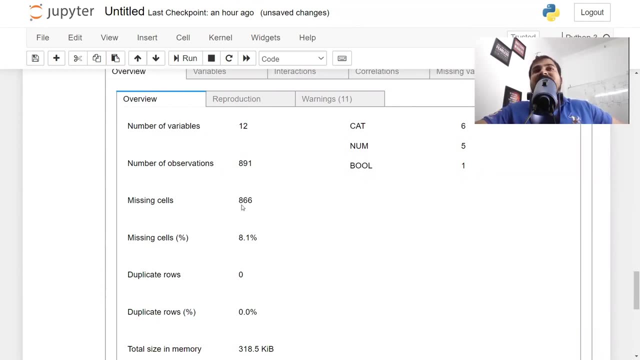 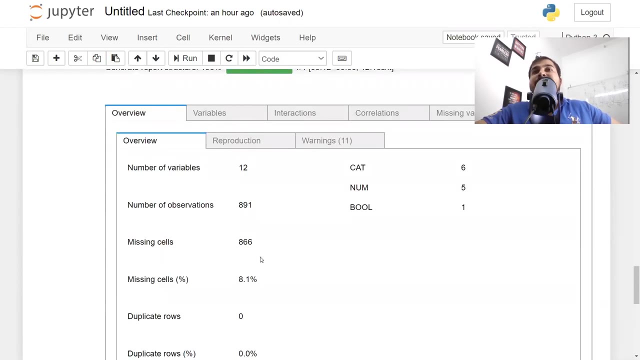 find out. the missing values are not so amazing. we have got over here. so the number of variables is 12. number of observation is 8, 9, 1. you can see the missing cells. how many missing cells are there? somewhere around 866. okay, missing cells is. that was somewhere on 8.1. percentage right. total size in memory. 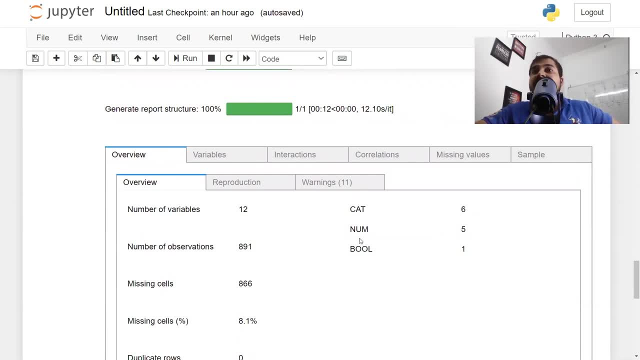 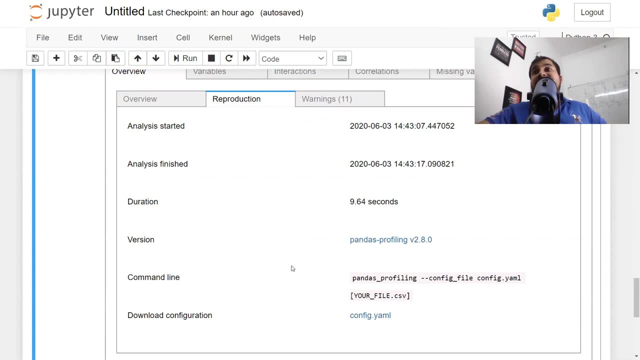 how many number of category variables are there? how many number of numerical variables are there? how many number of boolean variables are there? all this information, nine point six, four seconds, it just took to do the complete exploratory data analysis. guys, isn't it amazing, you know. so, here with 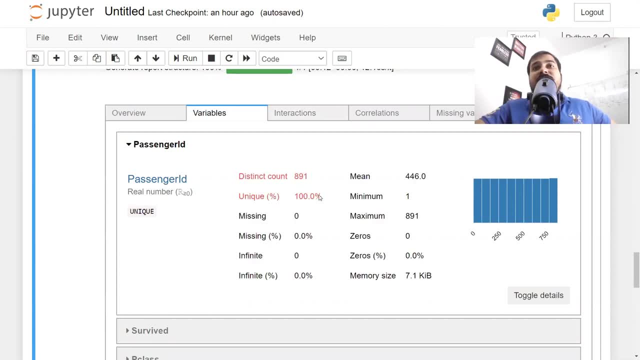 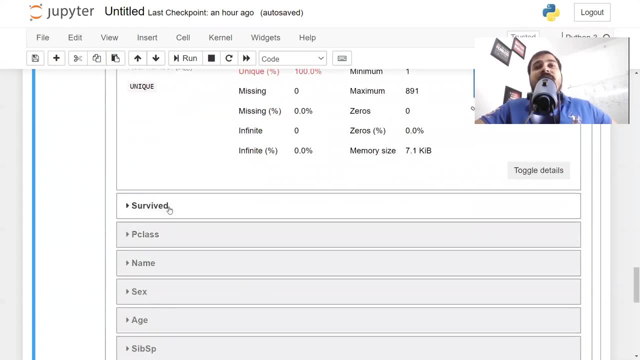 respect to the number of variables. you can see the number of variables is. you can see that I'm having district count of eight nine. one unique value is hundred percent. missing value is zero. and this is how the distribution looks like. mini mean, minimum, maximum, zero, zero. all values are there. similarly, with 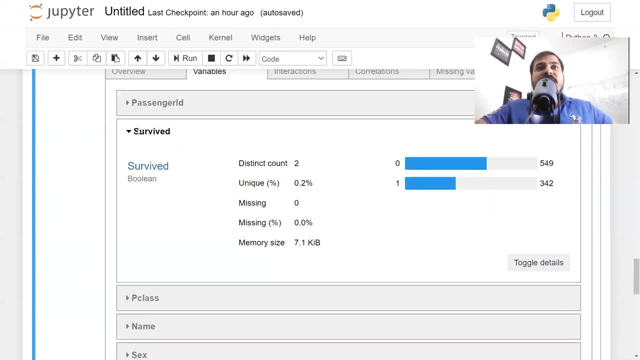 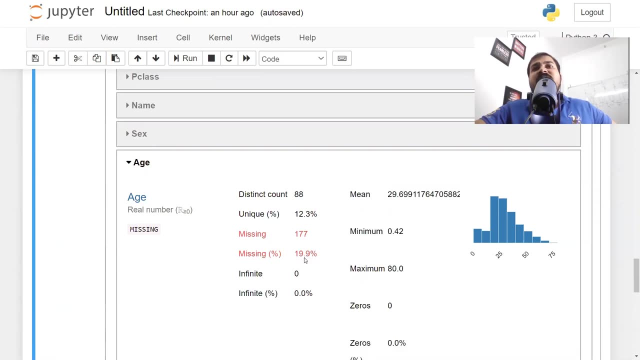 respect to survive. okay, all this information, you can check it out. I'm just going to go to the missing values. in age we have a lot of missing values, you know. we have somewhere on one seven where missing percentage in nineteen point nine, you know. so we can actually see that we also have something like 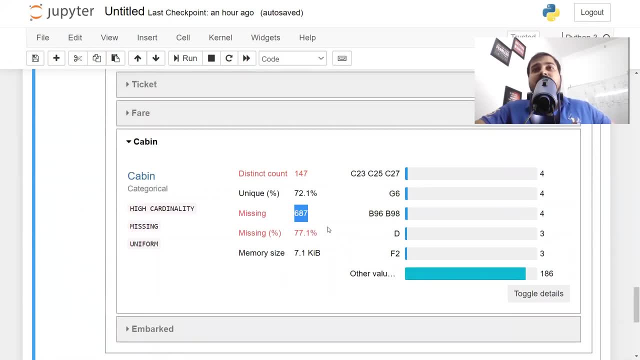 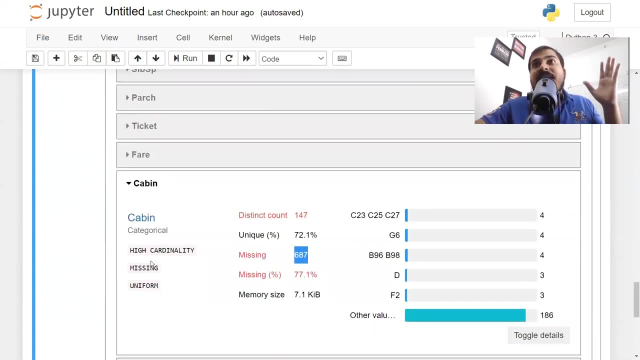 cabin in cabin also, we have a whole number of missing values right. so this missing values is basically saying us what are the missing values over here that is also present. it is also saying that, okay, it is a, it is a high card in our IT values. you know, it is a high cardinality. 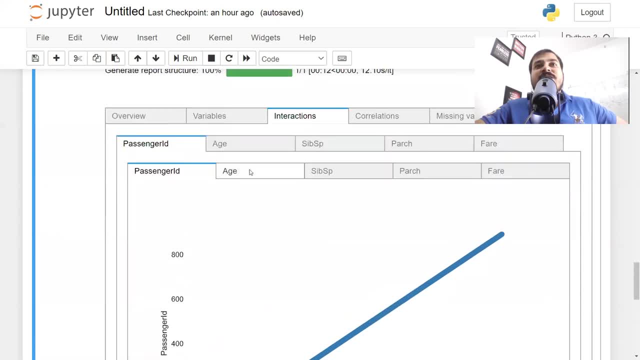 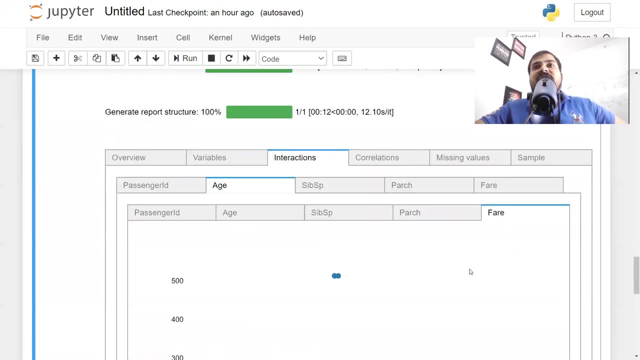 feature so that information is also there. interaction: you can see interaction with respect to passenger ID and age. suppose, if I want to see age and sibling spouse, if I want to see age and fare, okay, if I want to see age and are. and if you have not seen my exploratory data analysis with respect to titanic data side, it is the videos present in the 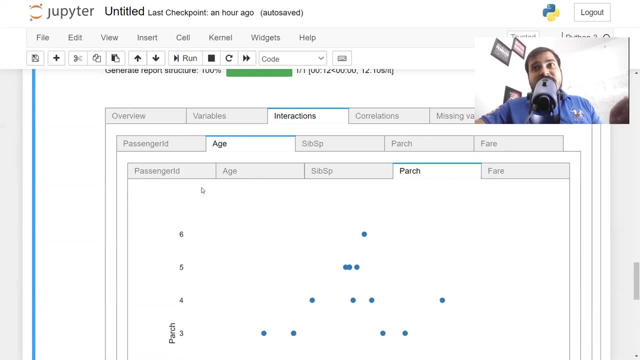 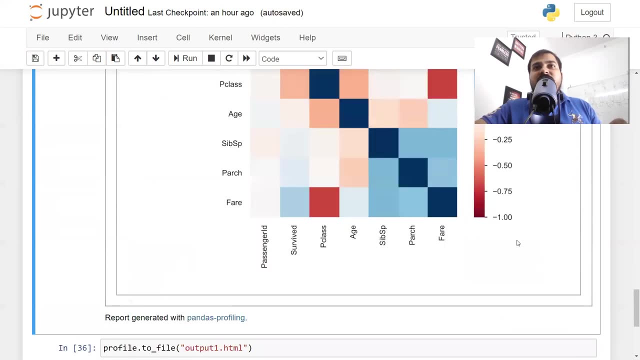 data analysis with respect to tightening data side. it is. the video is present in the complete machine learning playlist. you can check that. okay, now going to the correlation, you have all the correlation over here with respect to all the features that you have over here and if you see this color, it is highly. 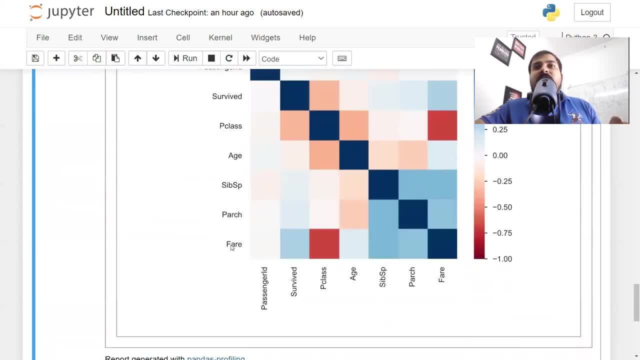 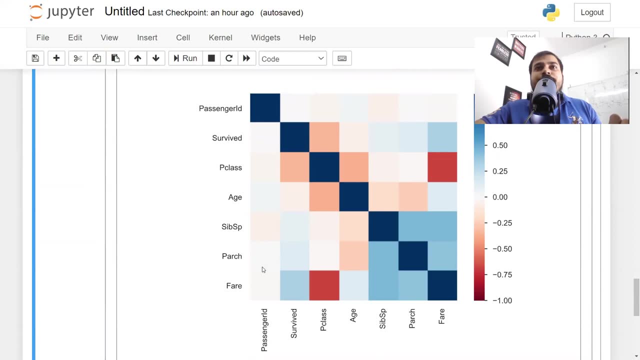 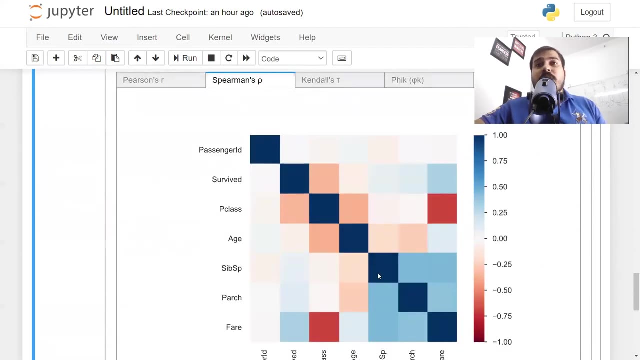 correlated. so if you, if you see this particular example, fair, and if you see sibling spouse, it is correlated somewhere more than 0.25. okay and different type of correlation you can actually find out from. okay, there were reverse inverse correlation, also considering this color that we have. so 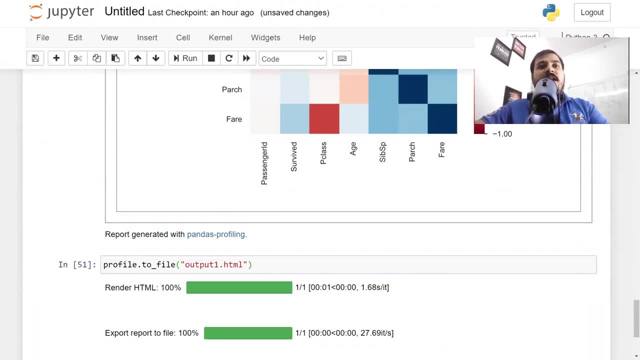 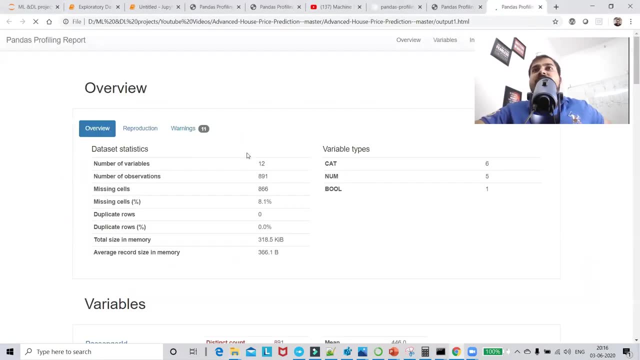 finally, I'm going to convert this into output one dot HTML, and what I'm going to do is that probably I'm just going to go to my folder now and I'm just going to click on output one dot HTML. so this is what output one dot HTML report is: 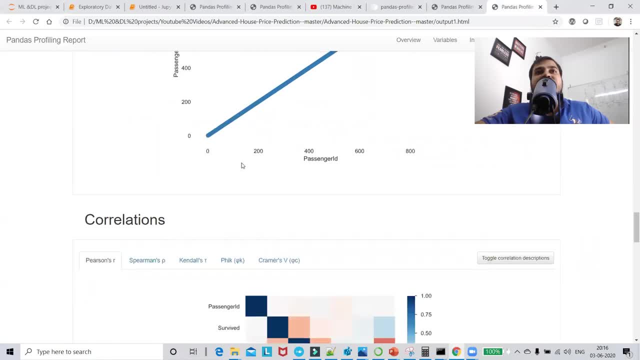 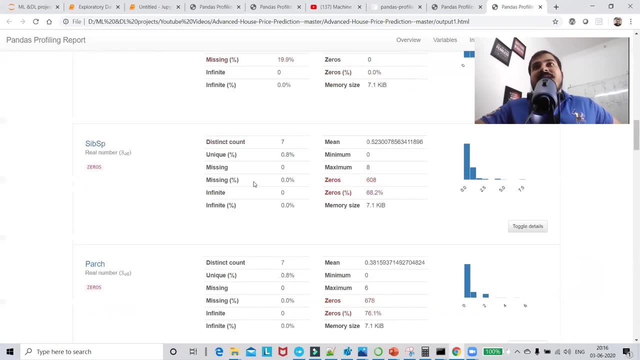 getting created. you can see all the same reports is being executed over here. now you can provide this particular report to any stakeholder that you want, right? so isn't it amazing? just tell me. just hardly within 10 to 15 minutes we were able to do it, but you understood. 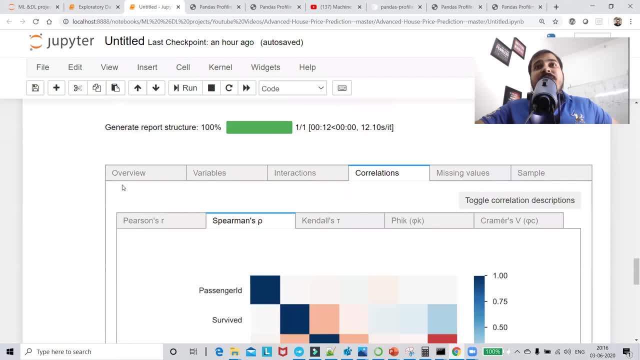 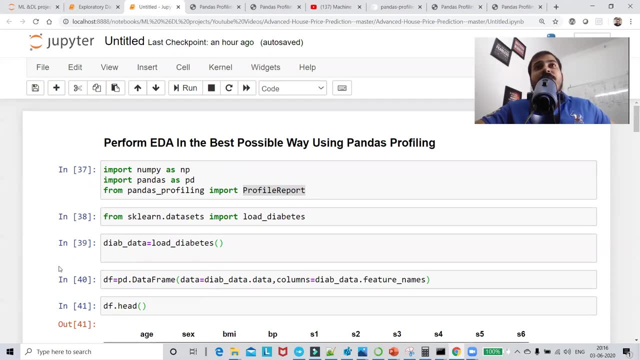 right exploratory data analysis when we are using pandas profiling, we are hardly able to just get it in five minutes, within five minutes. I hardly think it took around the five minutes, you know. so all these particular values, all these particular reports, will be attached in the description of this particular video. 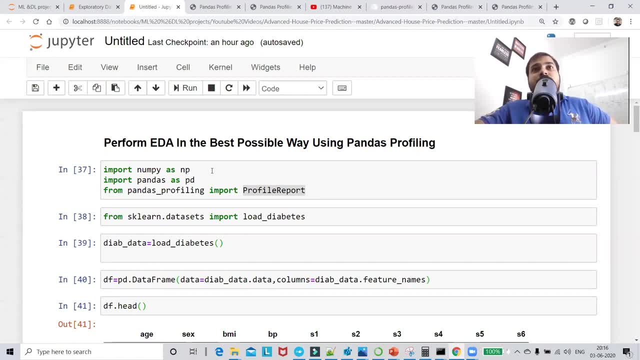 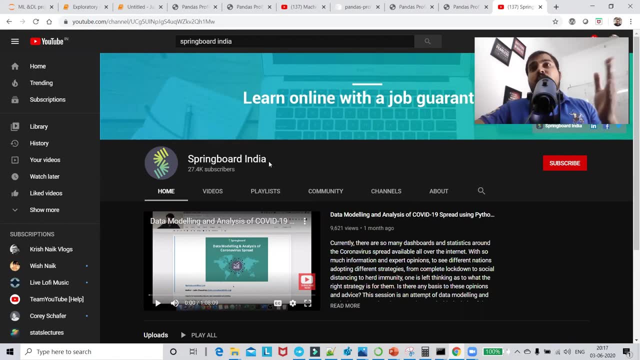 in the github, so please make sure that you download it from there. so, guys, if you are looking for career transition advice to our data science, please make sure that you go and watch spongebobcom. Thank you very much for watching this video. I hope you liked it. please do. 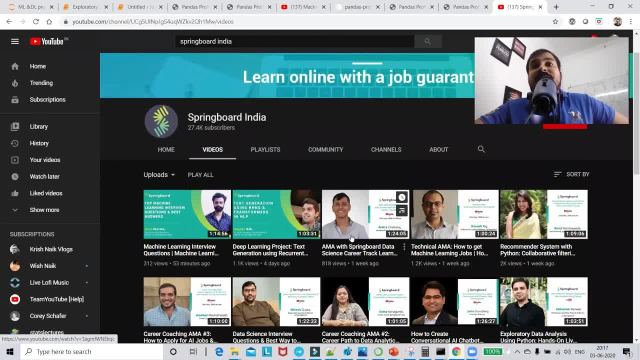 subscribe to my channel. if you have not already subscribed, I'll see you all in the next video. have a great day, thank you and all bye. bye.